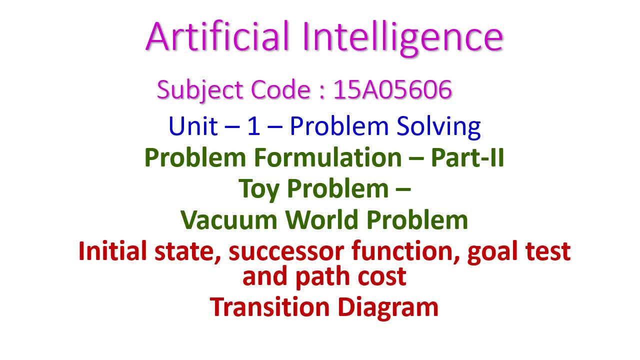 hello friends, welcome to artificial intelligence class. and here we are going to see some tie problems and in this video we are going to learn the vacuum mold problem, okay, and we are going to derive the initial state, successor, function, goal test and path cast of this vacuum mold problem and finally, we try to draw this transition diagram of the same problem. 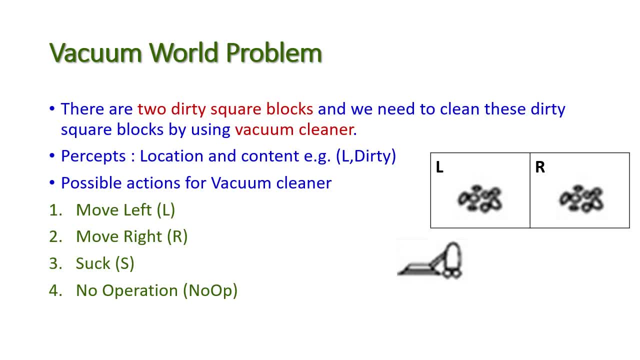 and vacuum mold problem. here there are two dirty square blocks and we need to clean these dirty square blocks by using the vacuum cleaner. here, vacuum cleaner is our agent. by using this agent, we are going to clean these square blocks. so two square blocks are there: left square block and right square block. 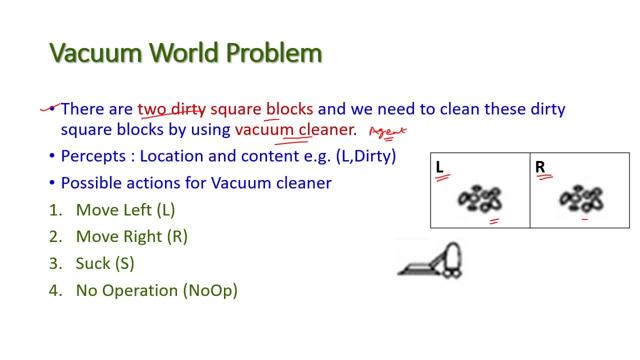 in both square blocks. blocks, Dirts are there, Okay, Both are dirty squares. And here the percepts, Percepts, What are the perception we are having? Location and content, Okay, Location is left or right and content, sorry, dirty or not. The content is dirty or not Okay. So these are the things. 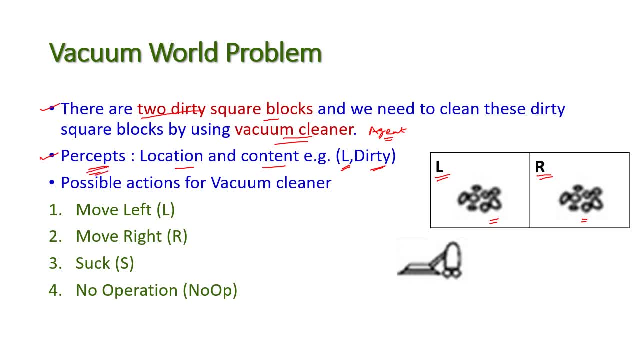 we need to perceive from the environment, Which is our environment. So this, the entire thing, are our environment. In the environment, we are having two square blocks left and right and both square blocks are dirty only, And the possible actions for vacuum cleaner are the first one is move left and second one is move right, suck and no operation. So these 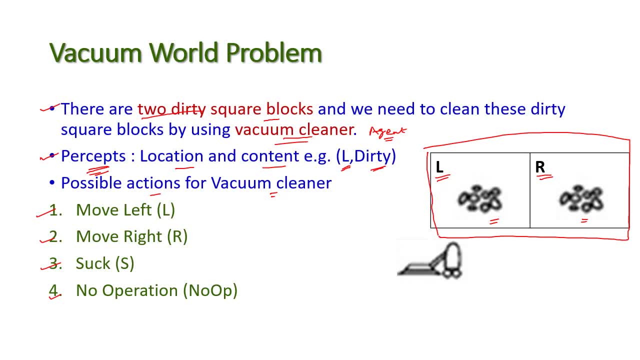 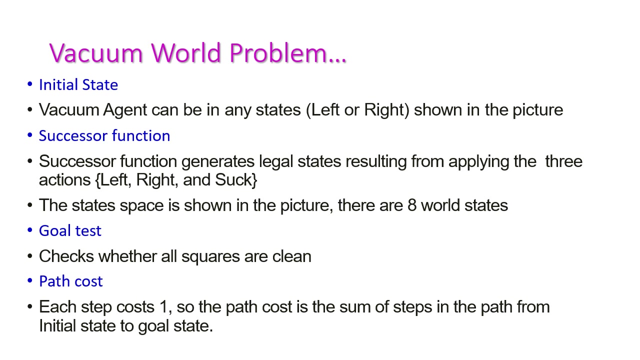 four are The possible operations of this vacuum cleaner agent. So this is our vacuum cleaner agent. What is the purpose of this vacuum cleaner? This is used to suck the dirt. Suck the dirt Right. And now let us try to derive the initial state, The initial state successor function. 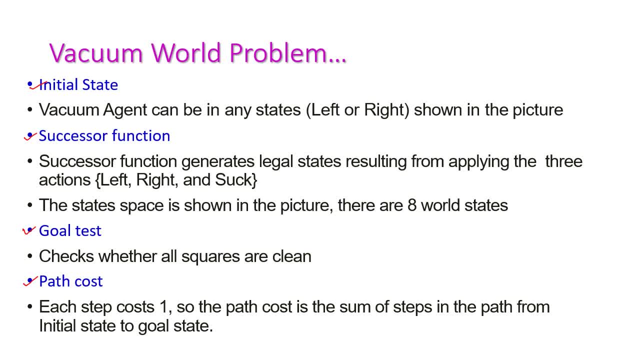 goal test and path cast. These four are very important components for solving any problem, Isn't it? So the first one is initial state. The vacuum agent can be in any state. That means left side or right side of the block. Okay, As shown in the picture. Already we 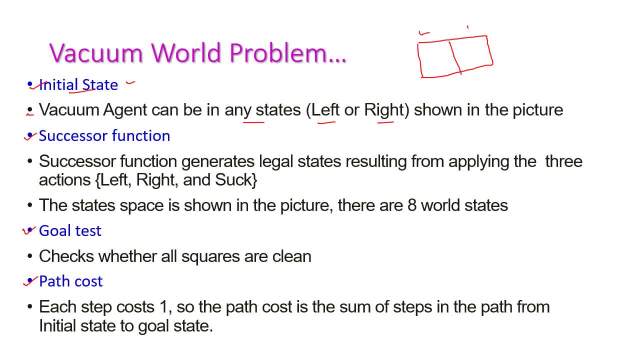 have seen this picture. This is left side and this is right side. Both are dirty. In the initial situation, our initial state is: the vacuum agent may be in the left side or it may be in the right side, Okay. And second one is successor function- Successor. 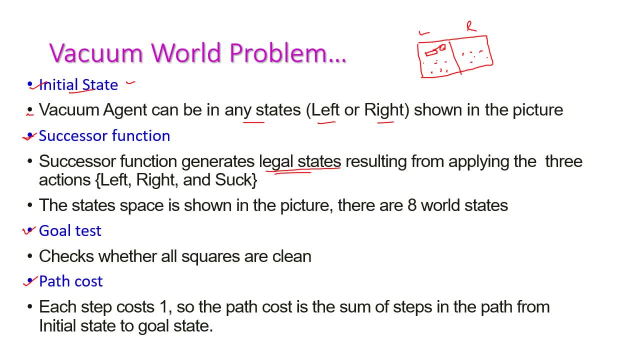 function: generate legal states resulting from applying the three actions. What are the three actions we are having? Move left, move right and suck operation. The agent may be move right and suck operation. The agent may be move left and move right and suck operation. 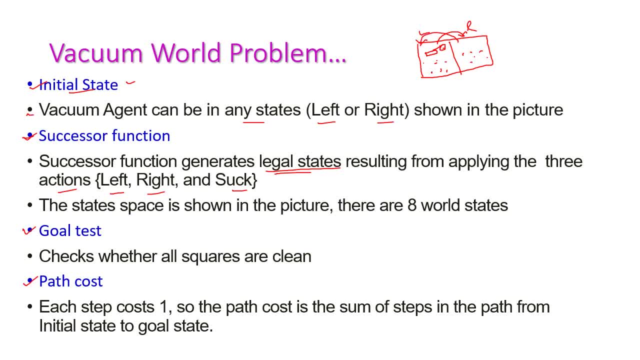 Right side, or it may be move left side, or it will suck the dirt. Okay, So these three are actions, possible actions of that agent. And next one is goal test. Goal test check whether all squares are clean or not. What is our goal? We need to clean all the squares. 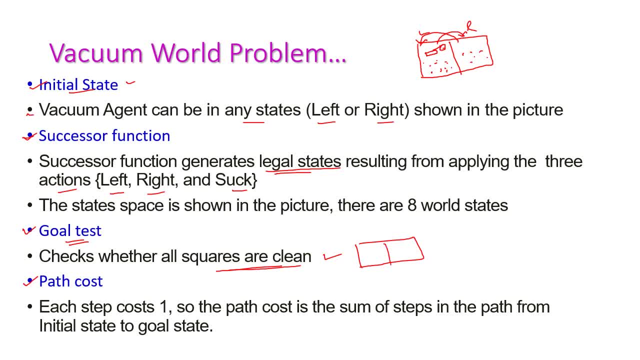 How many squares we are having? Only two squares. Two squares should be clean And next one is path cast. So here, each square should be clean. So here, each square should be clean. Each step cast is one. So they didn't give any step cast, So initially we can take one. 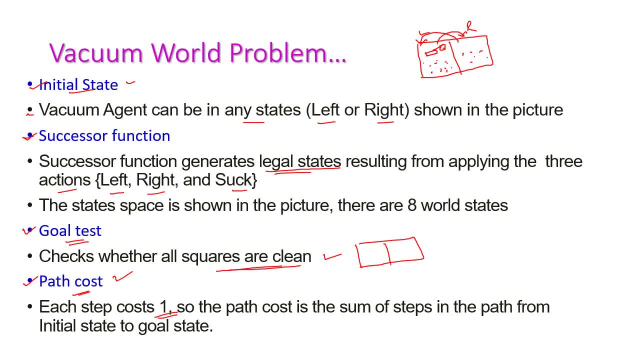 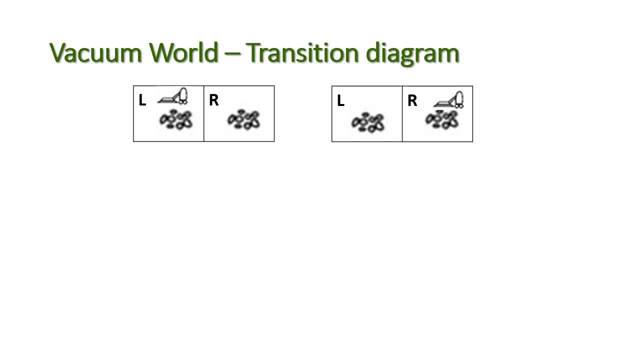 as our step cast for all the actions. So the path cast is sum of steps in the path from initial state to goal state. And now let us try to draw the transition diagram for our vacuum mold problem. here We are having two blocks and three actions, So total possible states of this particular. 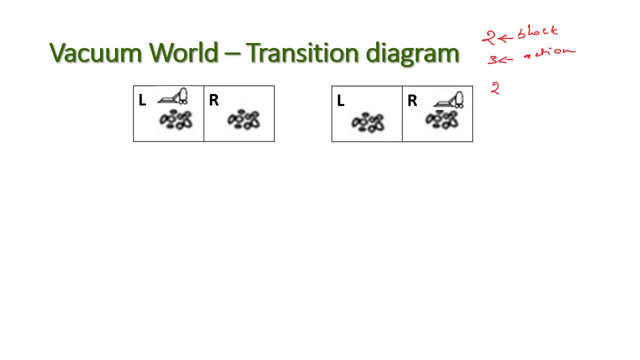 problem is 2 power 3.. Totally, eight blocks will be there. That is, eight states. States will be there And let us take this is our initial state. Okay, This is our initial state. So in the initial state, vacuum cleaner is in the left block And left block is dirty. 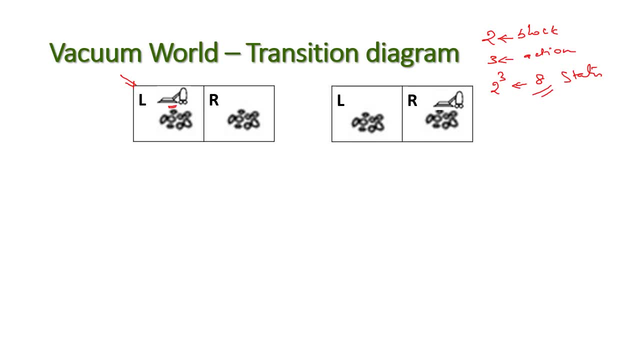 Right block is also dirty. Okay, Now, what are the possible actions there for this vacuum cleaner? It may move right side. So if the vacuum cleaner move right side- and this is our and this is our state, Okay, The vacuum cleaner moved to the right side, It may move. 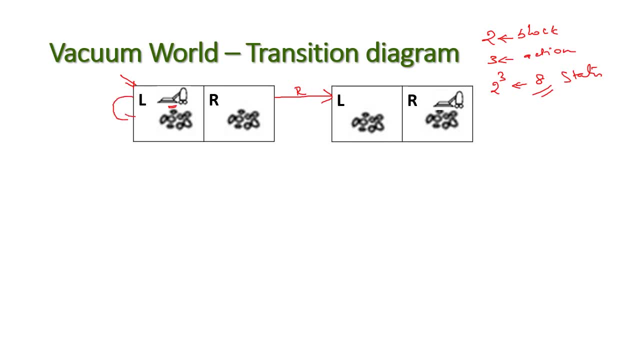 left. It may move. left means no operation, Because already the cleaner is in left side And it may do the suck operation. If it do the suck operation, Yes, Okay, Yes means suck And right side is dirty And left side is clean. Vacuum cleaner will clean this left And this. 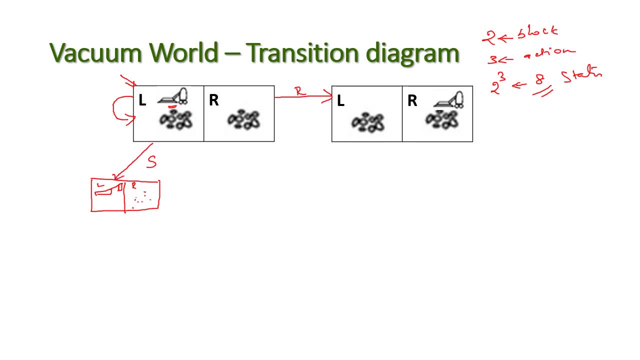 is left. Okay, If it performs suck operation, It may move left. It may move left, It may do the suck operation. Our state will look like this And next: Okay, What are the possible actions for this vacuum cleaner? now? It may move right side, It may move right side. So 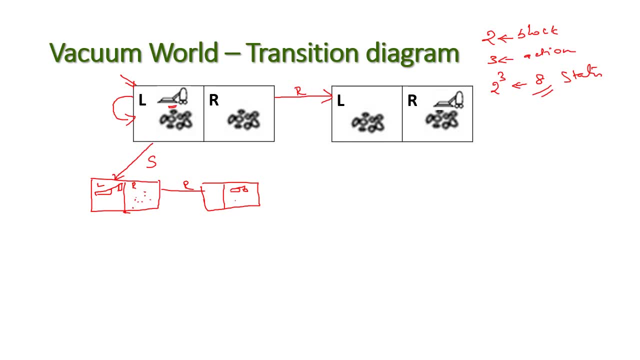 vacuum cleaner will be there. Right side is dirty, Okay. Or it may move left side. There is no operation because it is already in the left direction, So it may move right side, Okay. So at this point the vacuum cleaner can perform suck operation or it may do the. 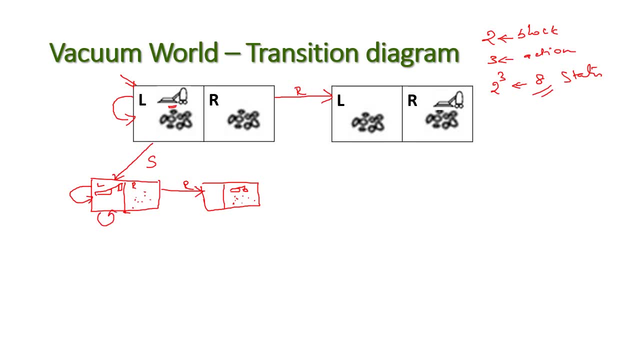 suck operation. Suck operation is also no action Because already the left side location is clean, Okay, So the only possible action is move right side, Okay. Now what are the possible actions for this vacuum cleaner in this state? So it can do suck operation or it may move. right, or it may move right. Okay, So this as surfing. Now there is no action, There is no operation prior to to to clean here itself or from the vacuum cleaner's work. Now, if you make of the vacuum cleaner is clean, Then there is no. 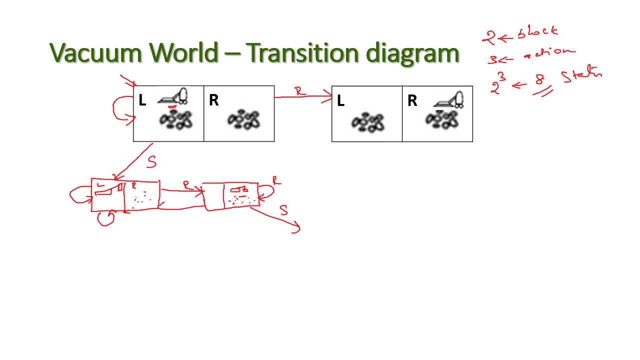 or it may move left, it may move left side. okay, if we go to left side, the left side location is already cleaned, so this is not required here. the only possible operation is suck operation. so if you do the suck operation, then both the locations, left and right, will be clean, okay. so this is our goal. this is our 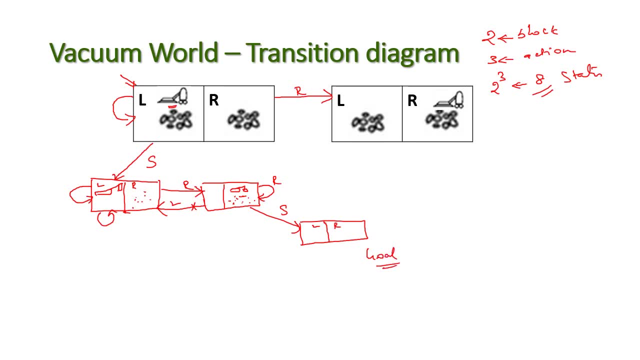 goal state. okay, when we start our initial state from this state, that is the vacuum cleaner in left direction, suppose if the vacuum cleaner is in right direction initially and that this is our initial state. if it is our initial state, then what are the possible actions? will be there, let us see all. 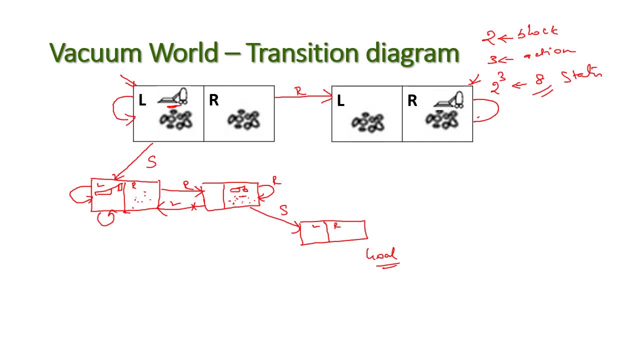 those things now. first one is move right. move right means this is already in the right direction, so no operation will perform and it may move left direction. if it goes to left direction, this will be the state okay. otherwise it will do suck operation, suck operation. okay. if it performs suck operation, the right side will be clean. 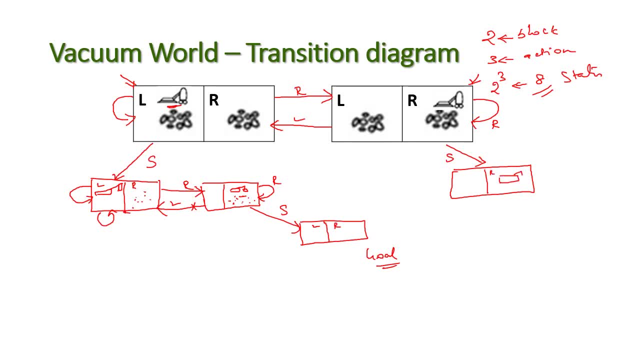 and the vacuum cleaner is in right direction. only left side is, as usual, dirty. left side is dirty, so this is the next state. what are the possible actions for this vacuum cleaner in this state? right move, right, move right will do no operation and suck- suck also will not do. 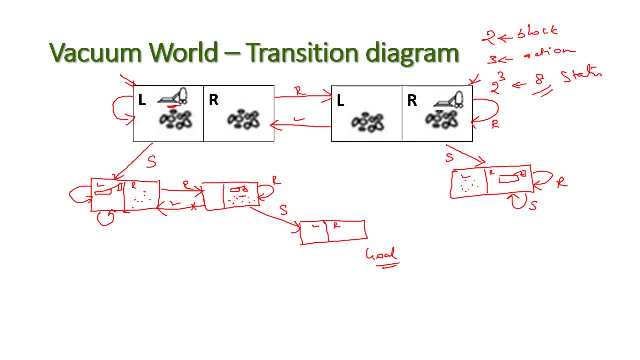 any operation because the environment is already clean and move left. okay, right side is clean, good. now, if we move left and the vacuum cleaner is in right direction, vacuum cleaner will move left direction, left side. left side is in dirty now, okay, so this is move left, right. okay, this is our new state. and now what are the possible operations for this? 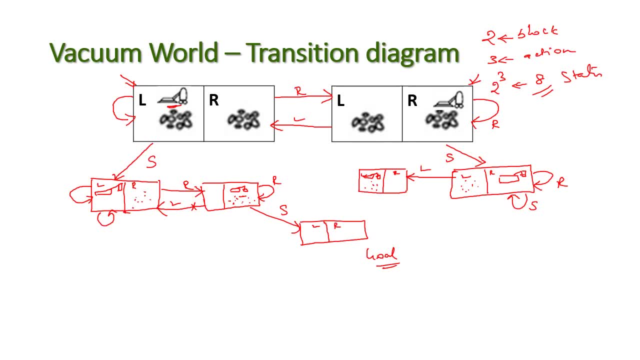 particular vacuum agent. it may move right direction, sorry, left direction, or it may move right direction, or it may do the suck operation left, right, okay. the agent is in left side, now here. the agent is in right side, now okay, and this is our cool suck operation. this is our.